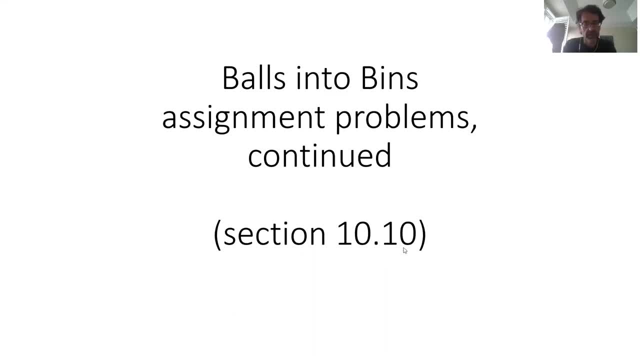 Hello students, This is an extra lecture on things that I didn't get to last Thursday And it continues the whole balls into bins treatment of taking a lens over all the counting problems as if everything was throwing balls into bins. So it will be a review of what we already looked at, but using this different length. 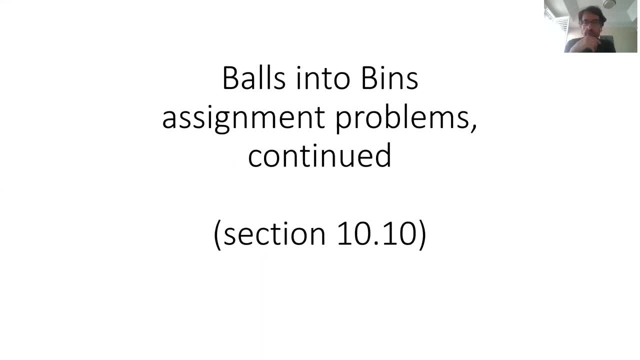 And also I will talk about the inclusion-exclusion principle, which we didn't cover And this will not be on the test. So I hope you will find it interesting and I'm sure you will find it useful, But feel comfortable that that part is not on the test, okay. 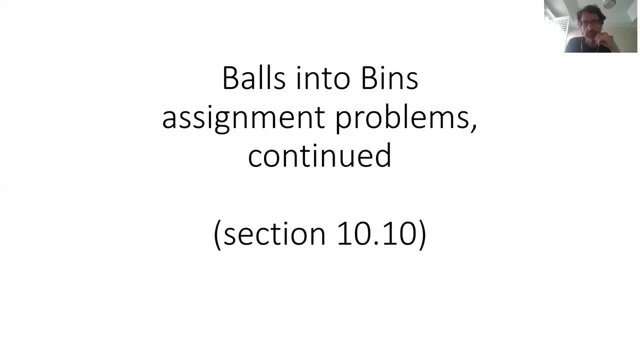 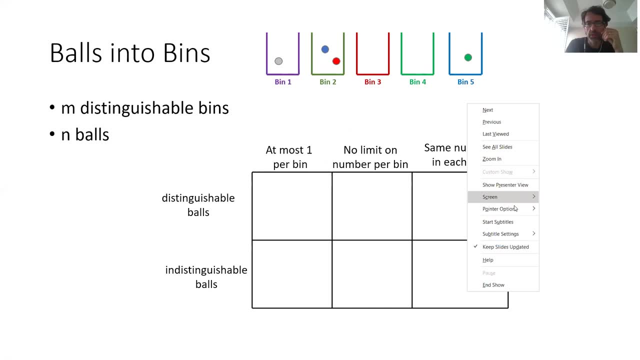 All right, so let's go into it. Let me get a better pointer here. Okay, so I'll make this quadrant of possible solutions To the general problem. So I have a bunch of bins M and a bunch of balls N which I'm throwing into the bins. 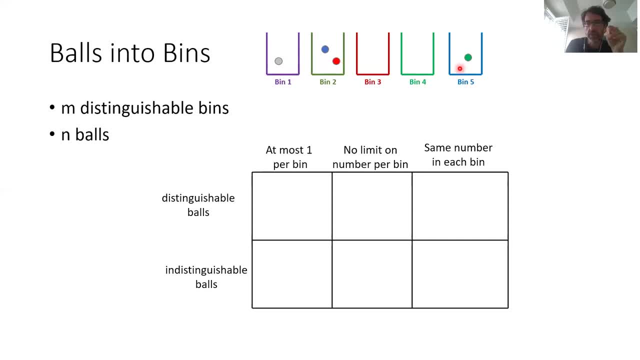 And every bin is different And balls in some of these versions would be distinguishable, like in here. Think of them as different color, every ball Or indistinguishable. All the balls are gray, okay, So it doesn't matter which ball went to bin one and which ball went to bin two. 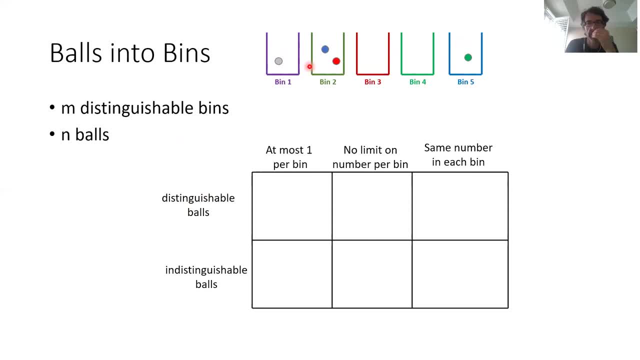 The only thing that matters is the count- how many? okay. So let's look at these counting problems divided in this way. So let's first look at this one. I have distinguishable balls, okay, So it's like this, okay. 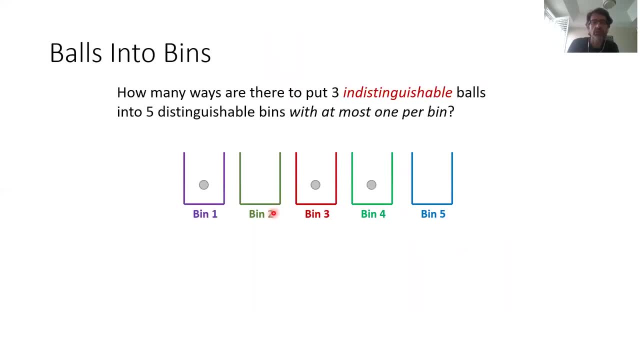 But I have a limit that, oh you know what. No, sorry, I will actually start with indistinguishable balls. So I have five bins- That's my M, And three identical balls- That's my N. How many ways are there to throw balls into the bins if you have the constraint that once you throw a ball into a bin, that bin is gone? 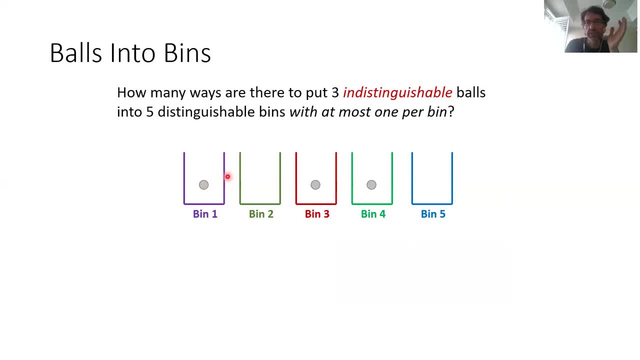 Like you cannot throw more And the balls are identical. Okay, So this is basically like I'm just selecting three bins, right, I just have to select three bins. That's the bins that the balls go to, So it's choosing three bins out of five. 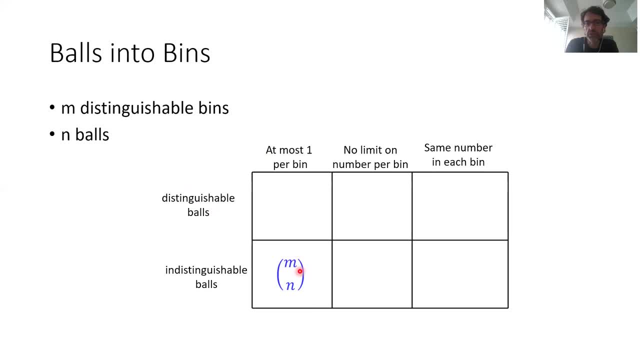 So it's five, choose three, right. So the general solution is M, choose N. If you have this constraint and your balls are all gray, okay, And you can only choose through at most one. So you can only throw three bins into a bin, right. 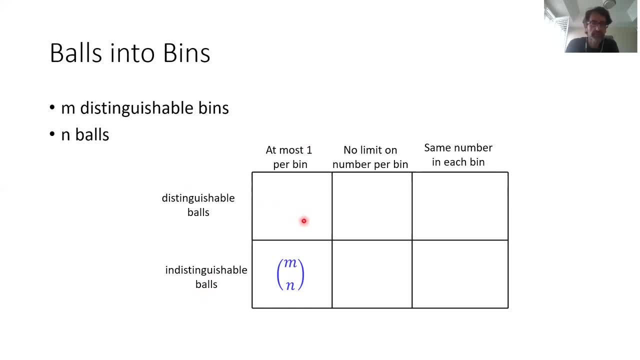 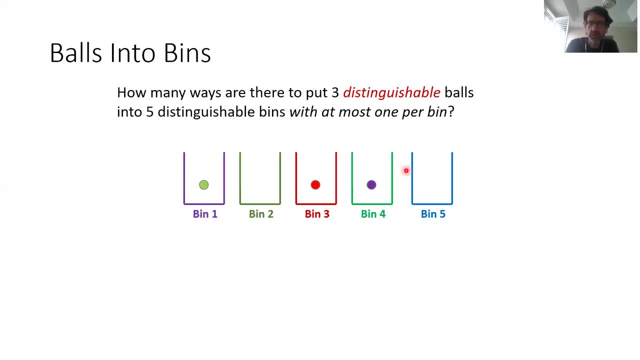 What happens if they become colored? So if the balls are not identical, Like so? Well, I can use the previous solution, Because let's just think of this as throwing gray balls into the bins And then permuting them And then suddenly giving them color. 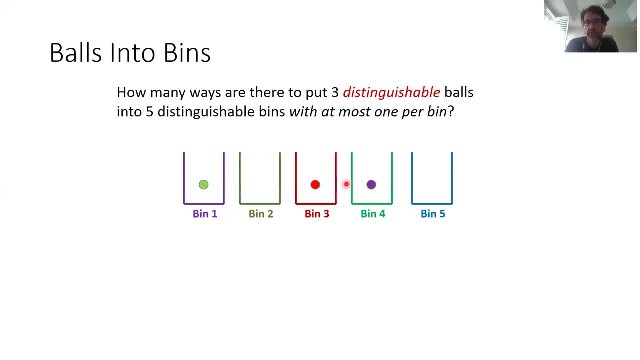 Which? how many ways are there? Three factorial right, Because it's the permutations of the distinguishable balls. now that all the permutations will count, right. So I'm choosing three out of five bins and then ordering the balls right Within them. 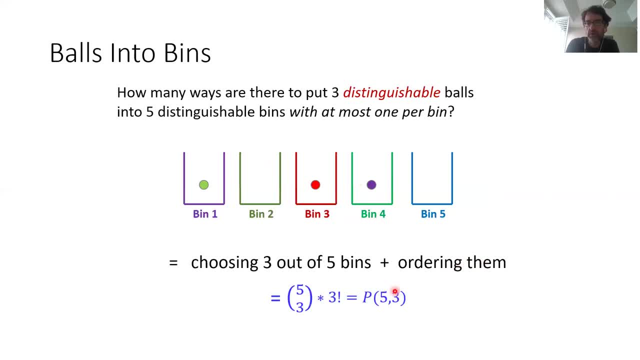 So three, So this will be five. choose three times three factorial, So it's a number of three permutations of the set of five, right? So if you squint your eyes, What are you choosing here? I'm choosing the bins, And how many? 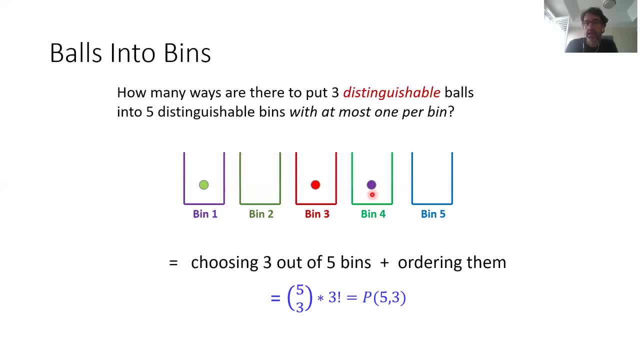 Three, Because that's how many balls there are, And if I just number the balls, then this corresponds to an ordered choice of bins. Like, if the green guy is my first ball, then this would be the first bin chosen. If the purple is second, then bin four is the next one chosen. 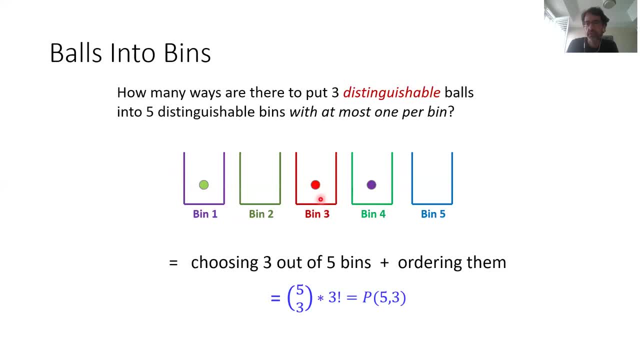 And if red is number three, then bin three is the next one chosen. So this, if you sort of think of this differently, of ordered choice of three bins, then you immediately get this formula right. But this is an equivalent way of thinking of this. 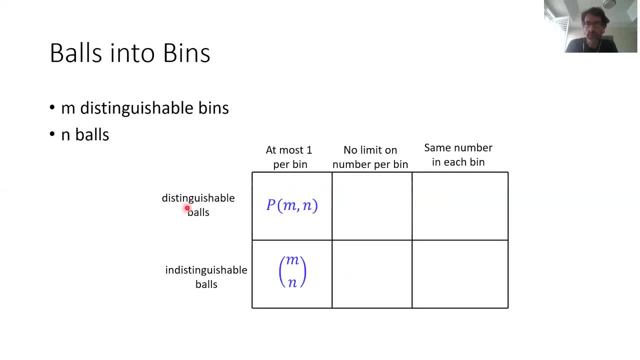 So if the balls are distinguishable, then it becomes an N permutation out of the N bins, Because I'm choosing N out of three bins. So I'm choosing N out of M bins in an ordered way, Whereas here I just chose them unorderedly. 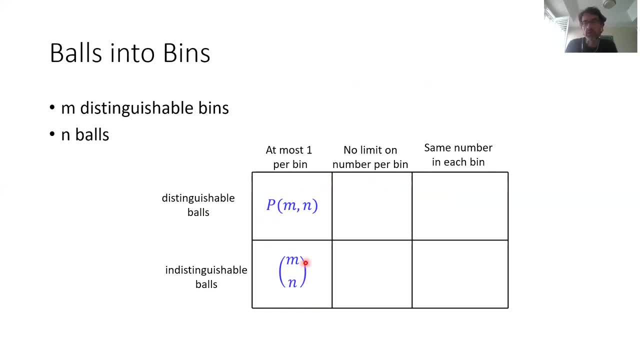 It's like a set that matters of which bins were hit, because balls are the same in this row. Okay, let's remove these limits and see what happens now. right? So this was under the first methods of counting, right, Like the N permutations. 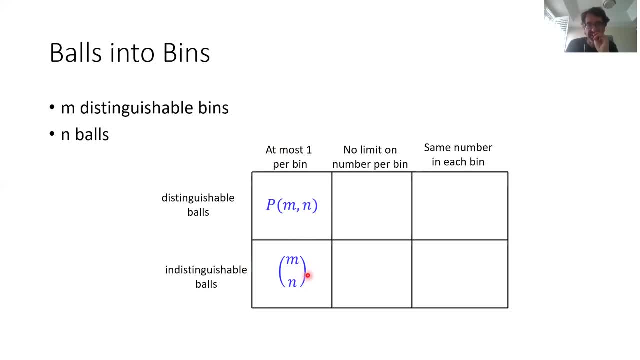 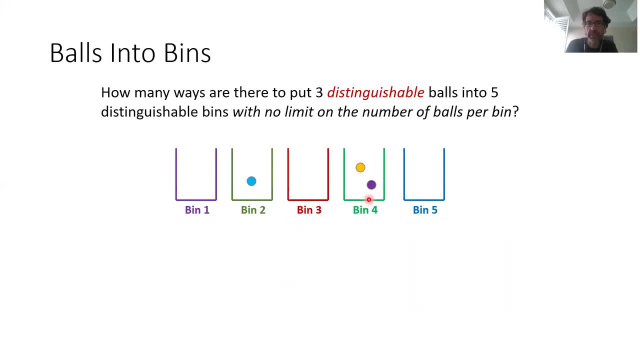 And combinations: Right Subsets. Basically, are this version of the balls into bin problem? What if I remove the limits? So let's look first at distinguishable balls. Right, The balls are colored And I'm throwing them into these bins. 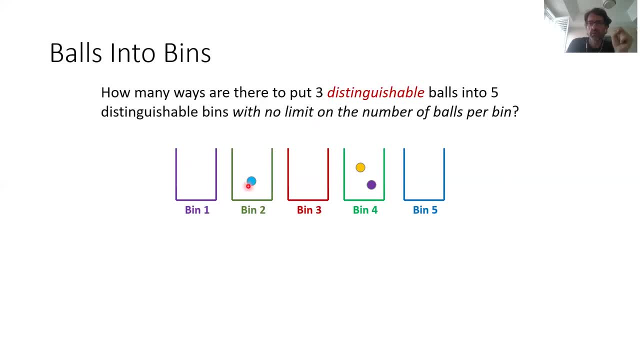 And now I don't have a limit. So basically every ball I throw it unconstrained, without any concern for other balls. So basically each ball is thrown independently, So it has five choices. So it's like this right: Five choices for every ball. 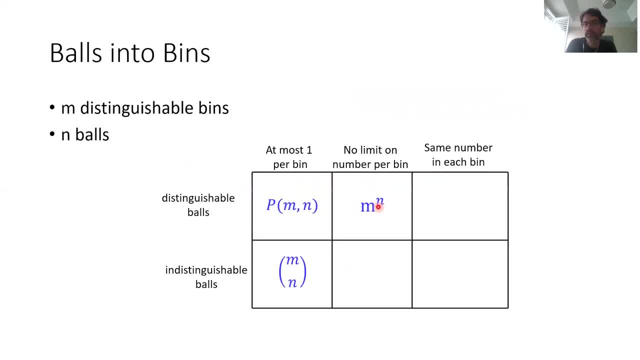 I have three of them, So this is the general answer, right? So, because basically this is the problem of having as many choices as balls there are, And the choice is always, for every ball, one out of M, So there's M choices per ball. 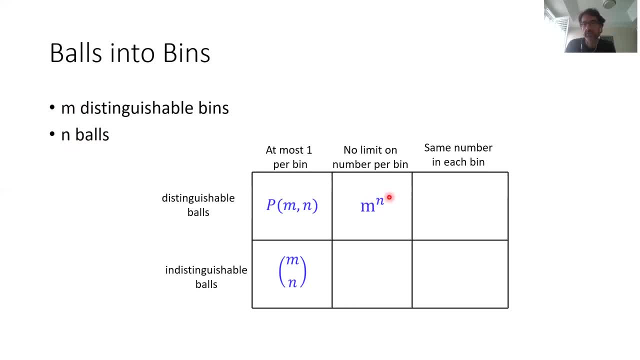 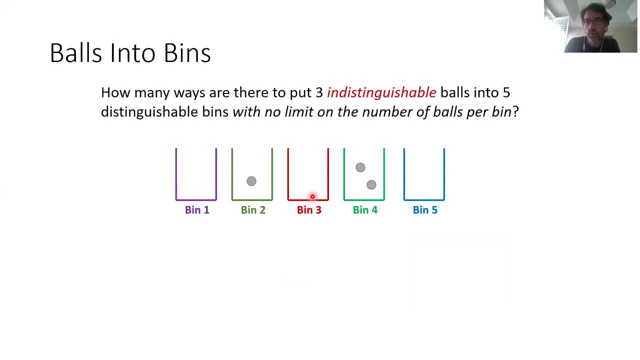 And you multiply these choices N times, Because that's how many balls you have. All right. What about if the balls now are become all gray Like so right, So you're throwing them without constraint, But they're all the same. 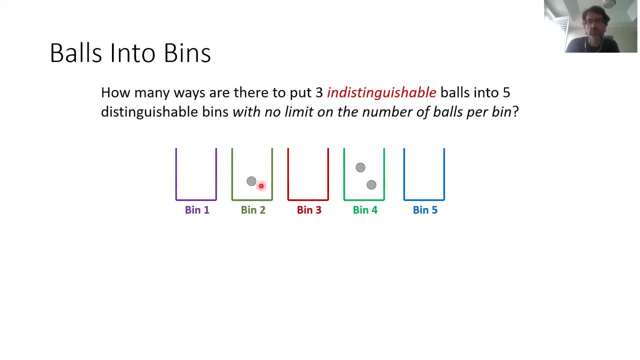 So it's as if each ball throw just chooses the multiplicity of the bin. Some are not chosen at all, Some are chosen once. This one is chosen twice. So what does this really resemble? Bins are your flavors And the balls are your donuts. 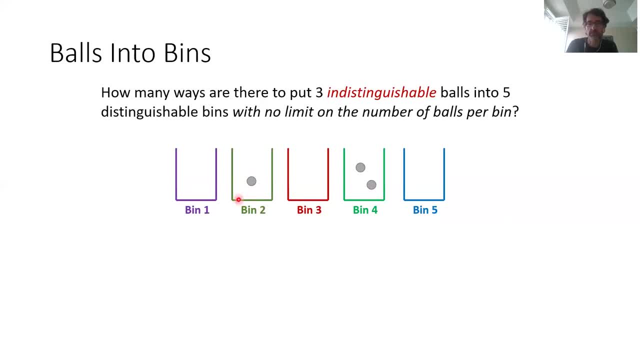 Right. So this is a choice of three donuts, of one of bin two type and two of bin four type. So it's choosing three items out of five categories I can choose. You know I have to choose three bins Because there's three balls. 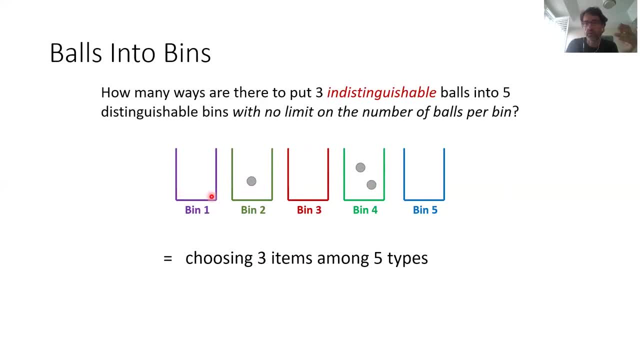 And I can choose them on any of these categories, Like three of these, Or maybe one of these and two of these. Right, That's what the balls do to the bins. So this is the donut flavor problem. It's choosing N items out of M. 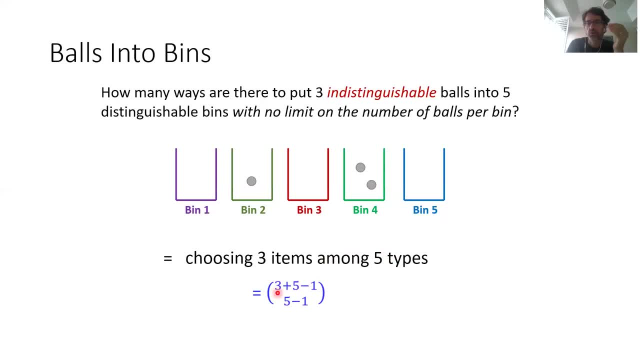 Types. So I take my items plus the types, Minus one. Choose the number of types minus one. Right, Because this is a guy. How do we do this? It's the number of bit strings whose total length is balls and bins and divisions between flavors. 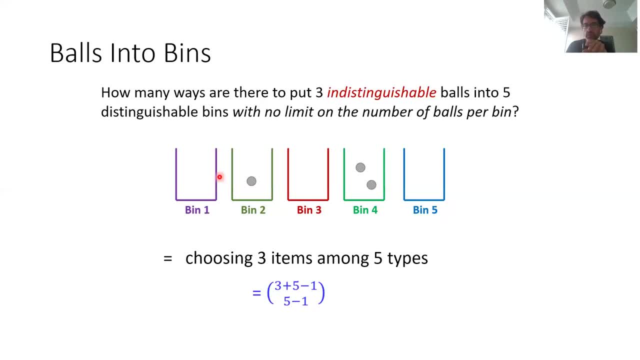 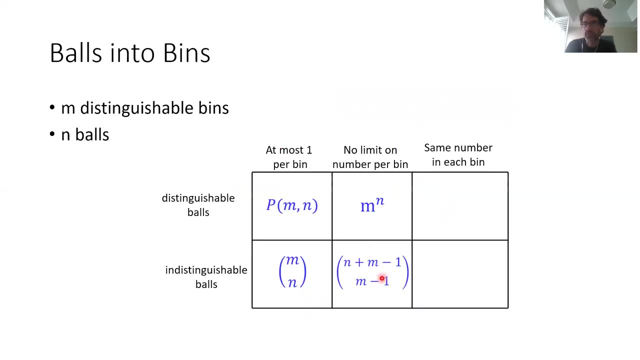 Right Between types Minus one, Because there is only four divisions Right, M minus one, Over either N or M minus one. This would be equivalent expressions Right. So this quadrant is the donut flavor problem Reappearing. 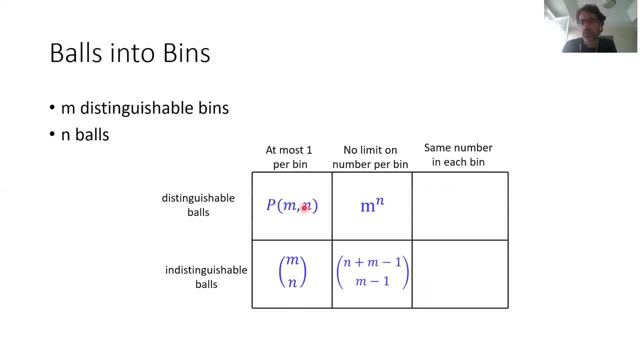 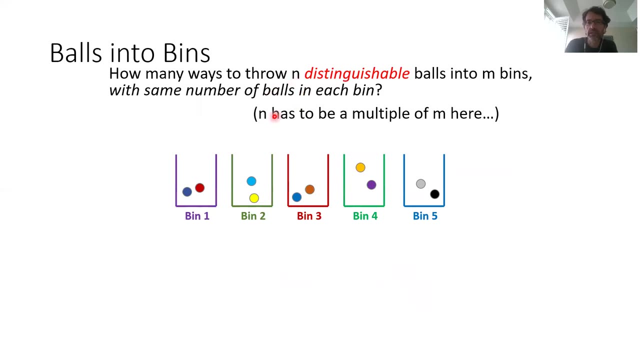 So what if I had this constraint, now that it's like a? Well, it's not a generalization, really, It's a different type of constraint. I want same number of balls in every bin, Okay, So now for this to work like, the number of balls has to be a multiple of the number of bins. 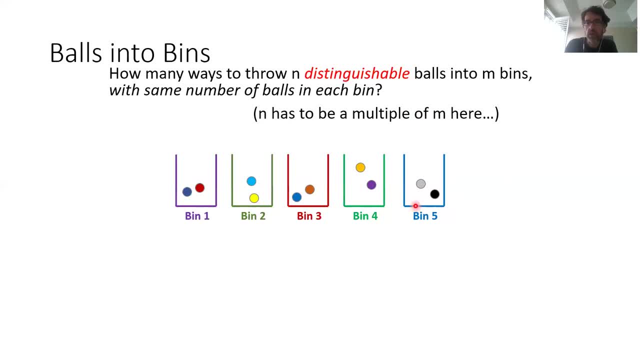 Right, Otherwise you could not place the same number. But balls are here distinguishable, So they're all different. Labels would say different number or different color, And the question is which color I'm putting where Right? So which would this? 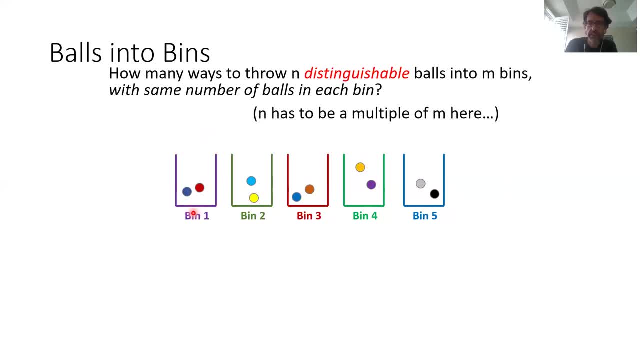 Again, it's one of our counting problems that we have seen. You can solve it by. This is How many of these choices there are. As many as there are permutations of all balls Right, Because I line them up And I can permute them. 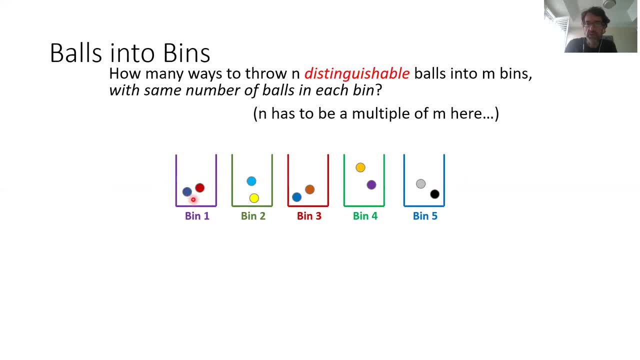 But not all the permutations matter, Because the internal permutations within a bin don't really change anything If I permute all of them so that all of them stay, but only these two switch positions, it's the same choice of placing these colored balls into bins. 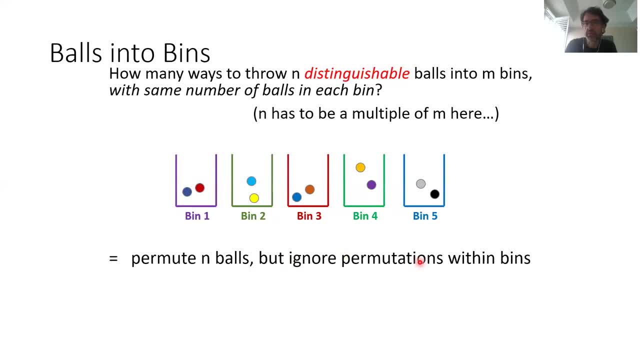 Right, So I have to divide, So ignore permutations within bins. I have to divide the total number of permutations of all the balls, n of them, by internal permutations within each bin. How many balls are in each bin? n over m. 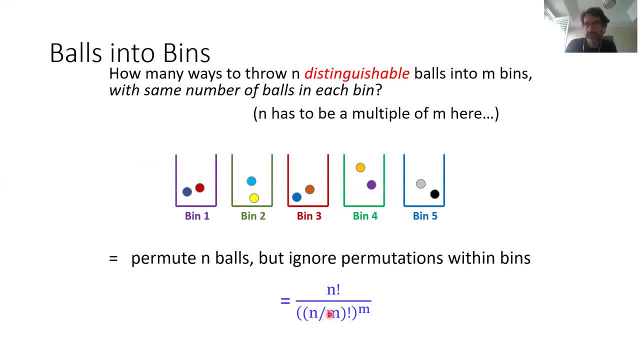 Right, The number of balls over the number of bins Factorial, because that's how many permutations within a bin you can make. And why do I raise it to m power? Because there are m bins, So I have to divide out These permutations. 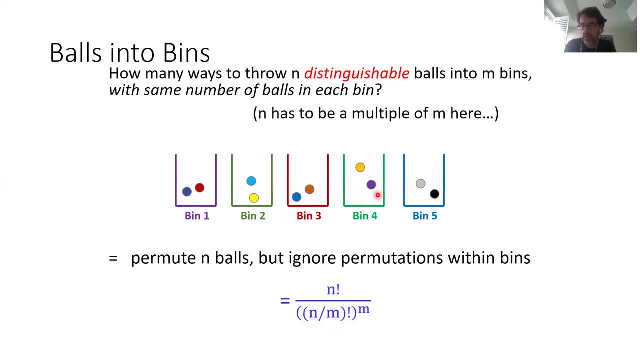 Internal permutations per each bin Separately, Right. So that's the k to 1 function that takes every permutation of n balls into only those permutations that matter, As in they ignore the internal permutations within a bin Of balls, within each bin. 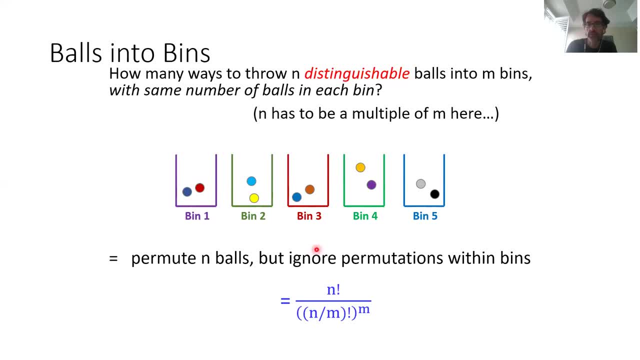 Right, That's how many you have to remove. You have to remove for that. And again, this is the problem. we have seen Right. So this is, We have seen this problem. It's the problem of ordering Right, But the internal permutation doesn't matter. 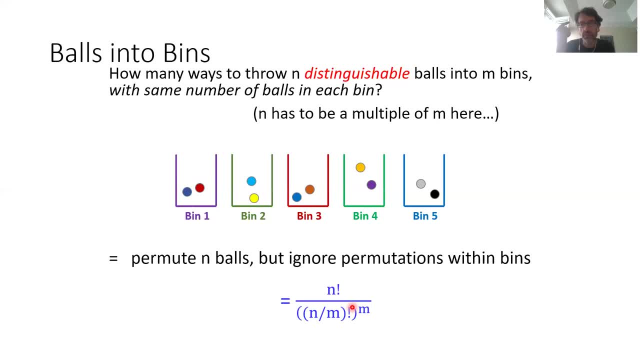 So where do we see this problem? How many words can you find with? Can you form Using the word Mississippi, Using the letters contained in the word Mississippi? There is a bunch of s's and a bunch of i's And p's. 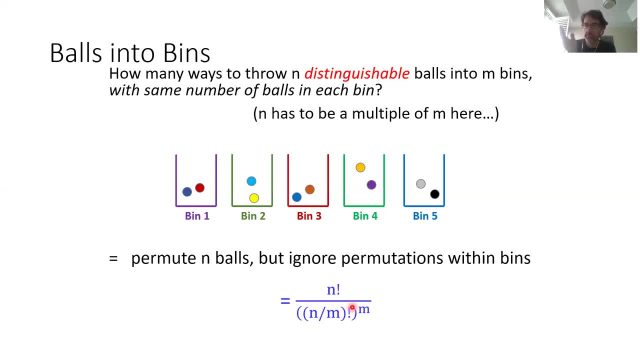 Right And you can permute all the letters, But then you have to remove the internal permutations of all the identical letters, Which are all the s's, All the i's, All the p's. These are the It's like this: 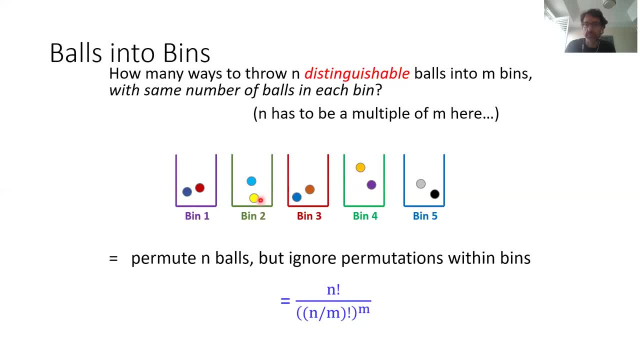 Because the internal permutations of these balls don't matter. Right, So it's an identical problem, Except as if, But only with the word that has the same multiplicity of every letter. Right, With Mississippi it's not one, And it would be hard to find a word like this. 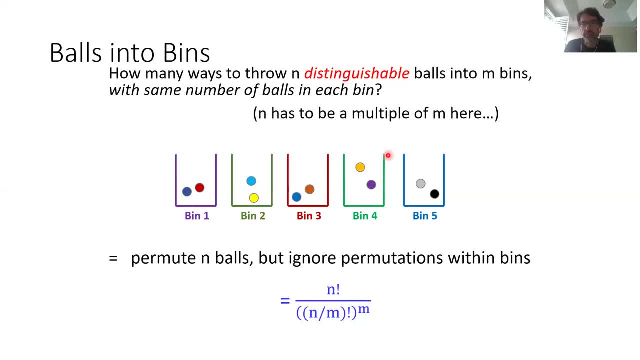 A long word that has only three letters And each of them at exact same multiplicity. All right, So. So that would form, you know, one of those quadrants in our diagram. And what if all of those balls are gray? 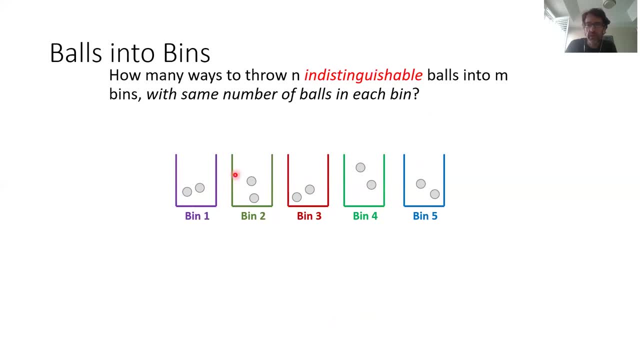 So what if all of those balls are the same And you still have this constraint That you have to place the same number in every bin? Okay, So that's a kind of a joke question, Because there are no choices here, Right? 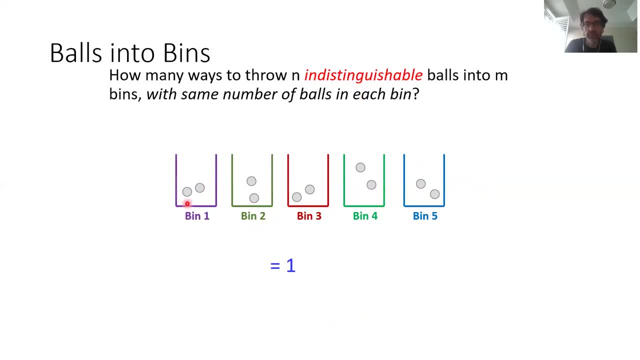 So, once There's no choice to be made, Every bin has to be filled with the same number of balls. It doesn't matter what balls, Because they're all the same. So what are the choices here? None, There is only one such arrangement. 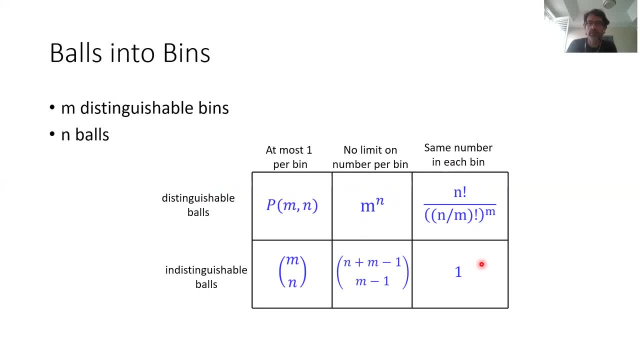 So these are the remaining quadrants, Right And now. you see, in this unified way, Maybe all, Or maybe there is one I forget about, But many of the counting types that we have seen. Okay, So I will Excuse me. 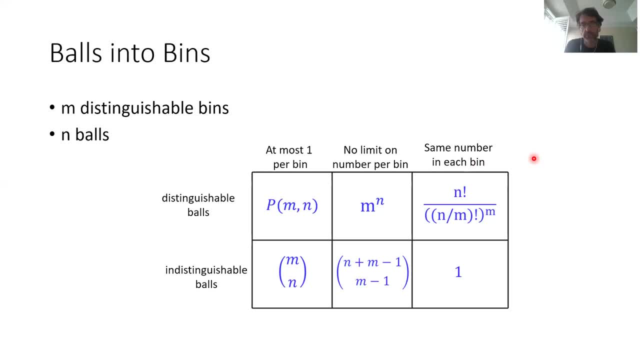 Now I will talk about inclusion and exclusion. Okay, Chapter Section 11. You can, you know, go away and close your ears and eyes if you really want to skip it now. But it's not long, It's not a nice. 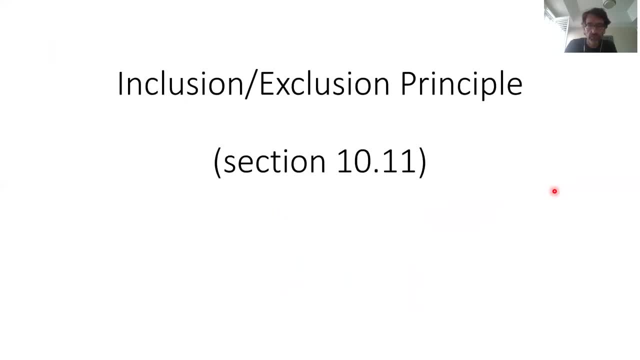 So maybe you want to stick around. Okay, So it starts with the sum rule. So we know that if you have to count all elements in a union of a bunch of sets, So you have some elements with some property A1, elements of type A2.. 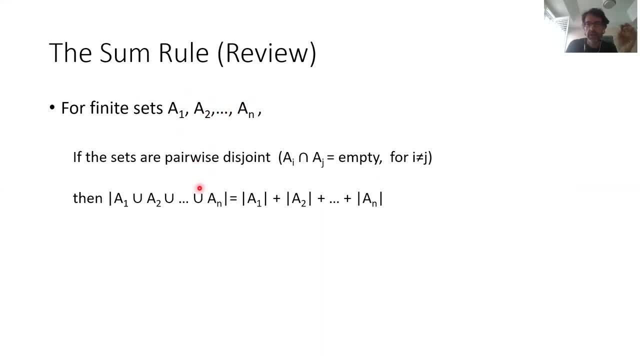 And you want to count all of them. Well, if there is no intersections between these types, you just count each separately and you add. But what happens if they are not pairwise disjoint? So if these sets are intersecting, That's the inclusion and exclusion principle. 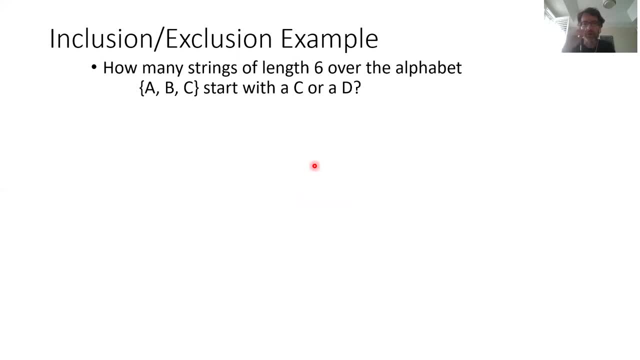 Okay, So let's give an example. You have strings of Words of length six over an alphabet with three letters- A, B, C- And you're told that they either start with either a, C or a, D. Okay, So you're counting really two sets. 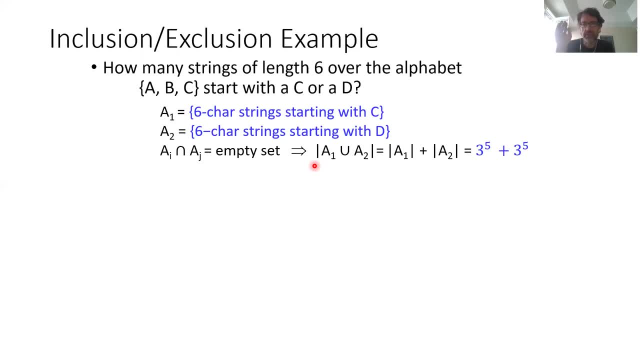 Set A1.. All six character strings will start with C And set A2.. Six character strings that start with D. Now you're in luck, because these two sets are independent. They cannot intersect. There is no word that starts both with C and with D. 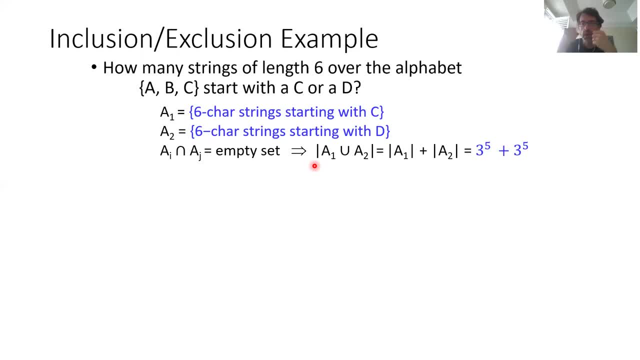 Right That such string does not exist. So nice, You count independently how many of such. You fix one character. The remaining five are free from this alphabet. So there's three to the five of these, And likewise there are three to the five of those. 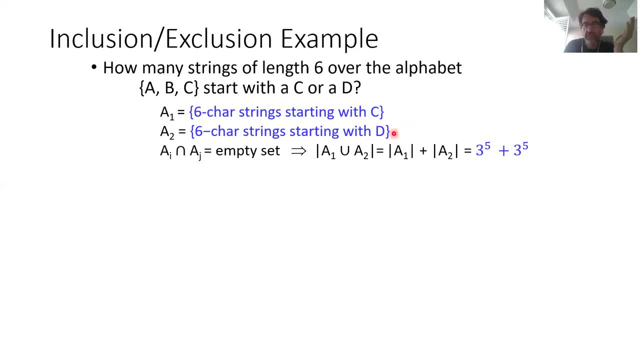 Because the truth, this character that you start with, is fixed. It doesn't matter what it is. So that's your answer. But what if I change the constraint? They start with C, They start with C or end with C, These six character words. 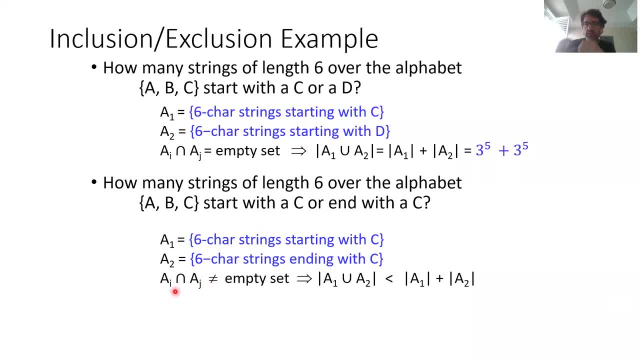 So now it's not so nice because they intersect. You can have strings that start with C and also end with C, So the size of this union is smaller than the two sets. It would be the two sets combined. right Added the cardinality of these two sets. 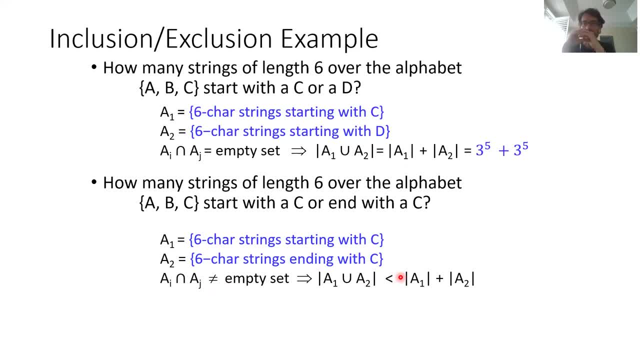 If they were separate. But if they are combined, well then, if you add, you overcount. You overcount those which are inside Right Of both In the intersection. But that's inclusion and exclusion. It's easy, You just subtract those which are in the intersection. 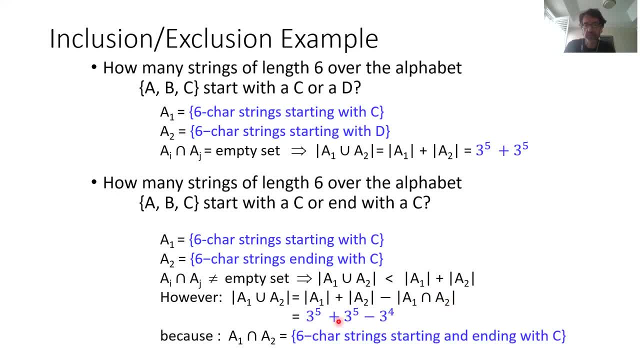 So let's see, Okay, So the answer here would be again the multiplicity, the cardinality of these sets we already established. And what about this one? Well, there is only this is a set. You have to kind of see what this set is. 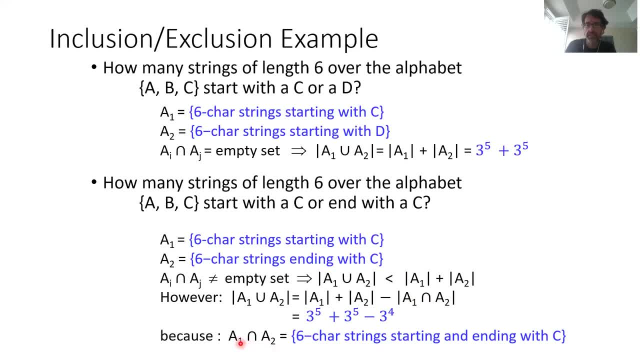 Right. Well, what is this set? It's a set of words that satisfy both constraints: Right, Because they belong into this and into this, So they satisfy both constraints. So these are six character strings that start with C and end with C. 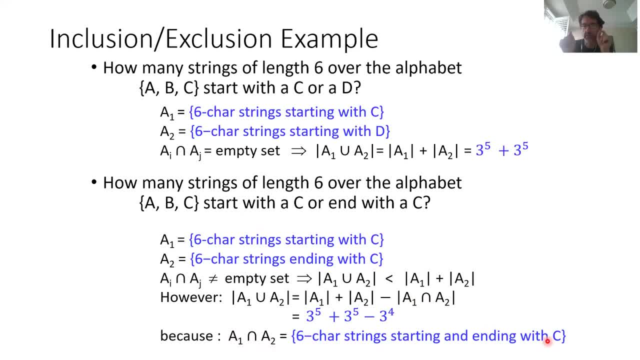 Well, but that's easy. So you fix two characters in a string. The first one is C, The last one is C. How many choices remain? Four, They are unconstrained. So this is the multiplicity, the cardinality of this set. 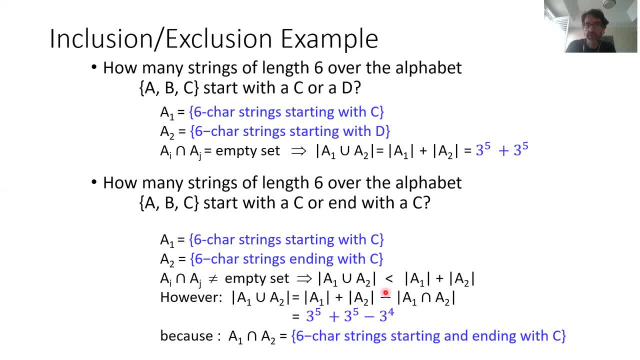 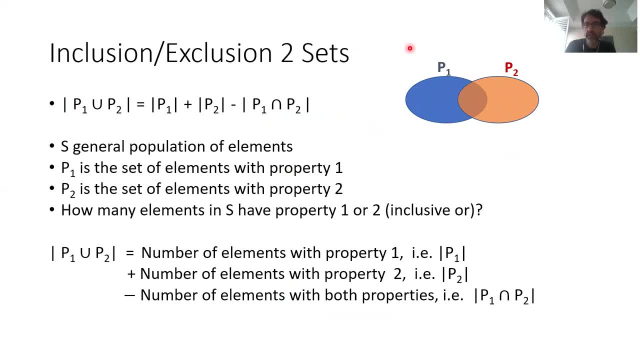 And you subtract it. Why is it? Why do you subtract? Well, it's easy to see on the picture. So the general formula is this: Cardinality of the union is the cardinality of set P1 plus cardinality of P2 minus the 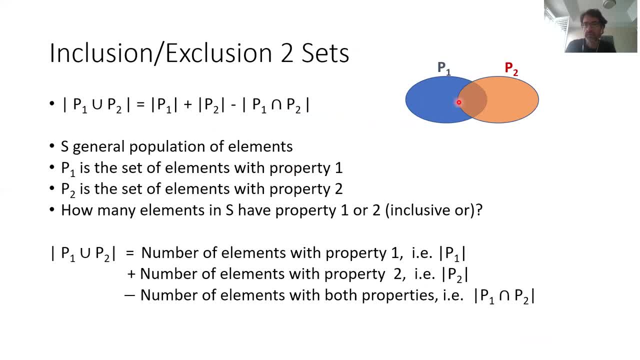 intersection, Because if you think of this right, You have to add everything that is purely blue, everything that is purely orange and the stuff that is both. If you just add the cardinality of P1 and cardinality of P2, you're adding these guys. 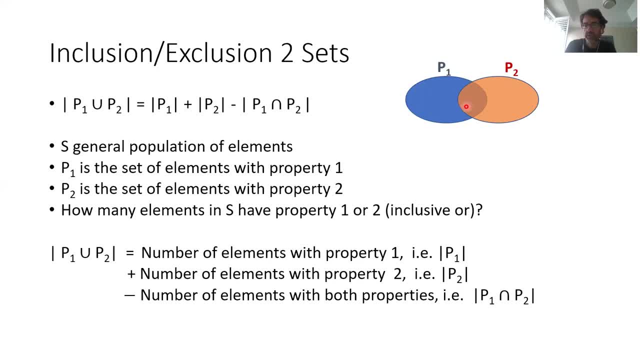 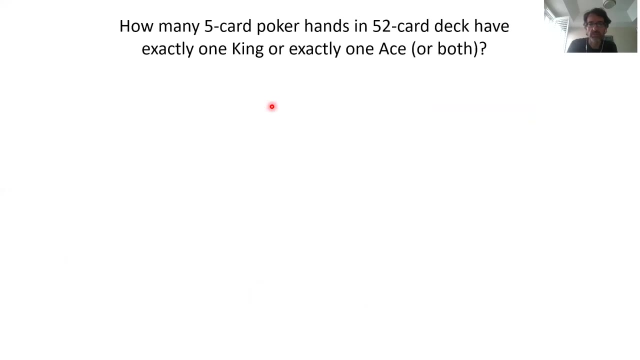 in the middle twice. So you just have to subtract them once in order. So the remaining is the blue plus once the mixed plus the pure orange. So this is the general formula that we used on the previous slide. Okay, Let's do another example. 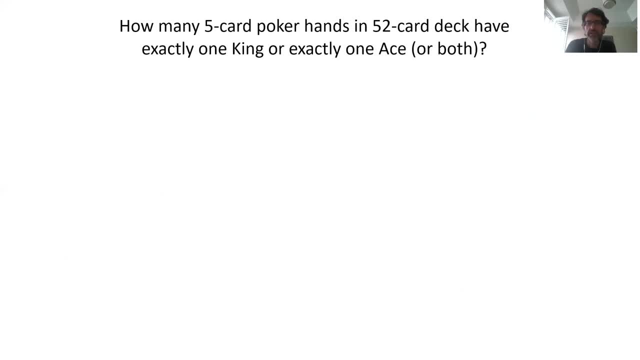 How many five-card poker hands in a 52-card deck have exactly one king or exactly one ace, Or both, Because not an exclusive, or Okay, Okay, So, okay. So let's look. So you have these two sets. One is five-card hands with exactly one king. 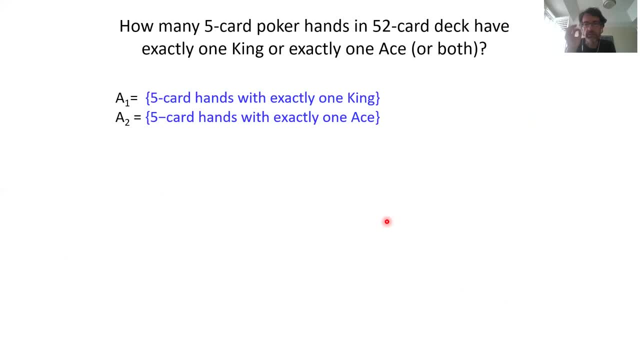 The other is five-card hand with exactly one ace And clearly they can intersect, right, Because you can have a five-card hand that has one king and one ace. So let's So you know that the you you can count those that belong to the union. 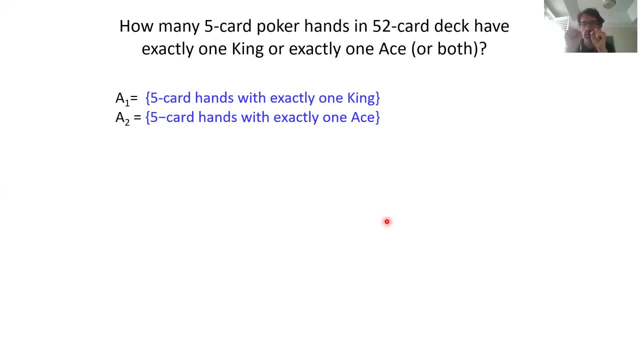 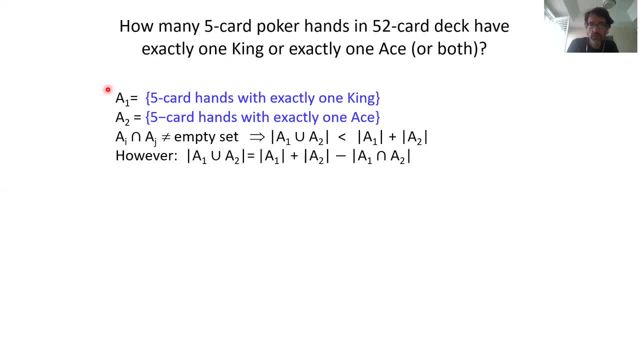 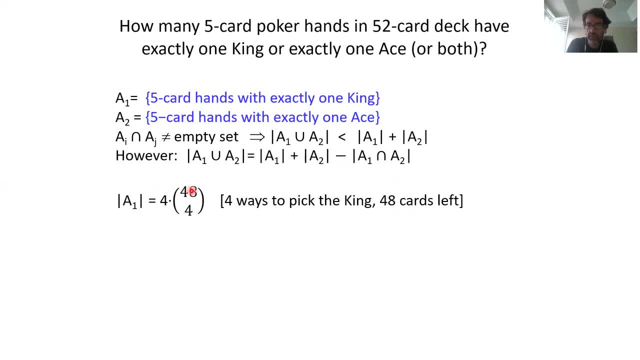 that's all. so you kick out four cards from the deck of c2 and that's where you choose your four. a2 is the same story, right, because it doesn't matter whether it's a king or an ace, it's the exact same um way of counting. what about counting this set? okay, so let's see what it is right, oh it. 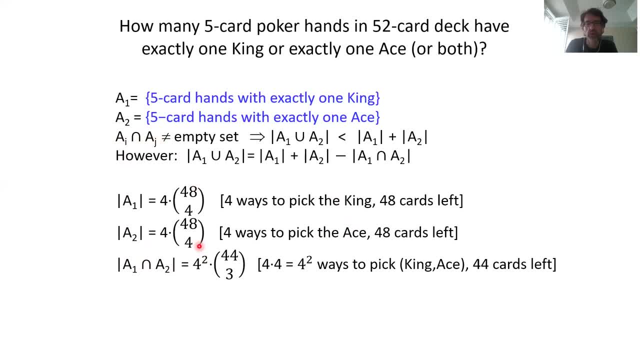 should be a1 intersection a2 here. all right, so the, the. what is this set? well, it's a set of cards that have exactly one king and exactly one ace. so you have to choose the king four ways, you have to choose the ace four ways and you have to choose the remaining three cards. 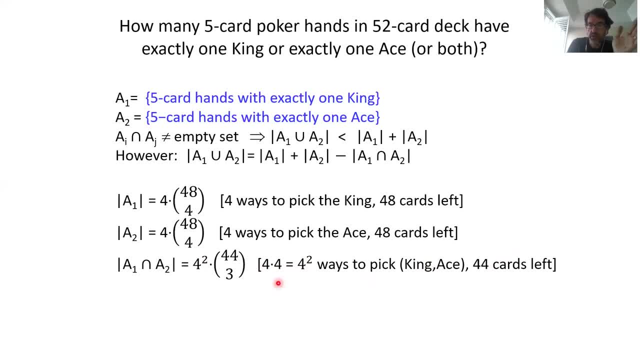 out of 44 because you kick out all the kings and you kick out all the aces. the remaining three cards cannot be either a king or an ace right, Because the constraint is exactly one king. In the intersection, the constraint is exactly one king and exactly one ace. 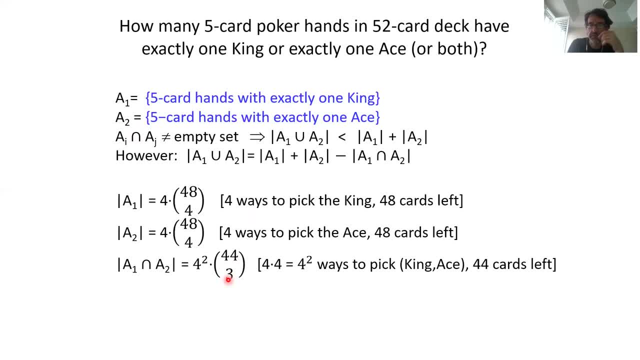 So there's 44-3 for the remaining cards, So don't do this too quick. okay, Again, I will not put this stuff on the test, but this is really good things to know, So you just have to be careful as to what are you now choosing. 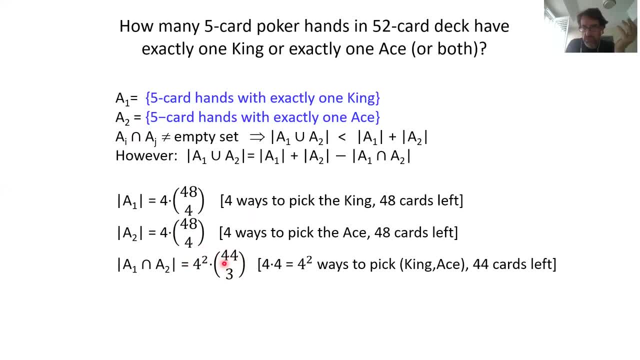 It is related to these, but it is an instance of a similar problem, right, But here, in this case, you're choosing from the reduced set. now, right? So this will be the. I mean sorry, this would be the particular answer using the general formula, which is this: 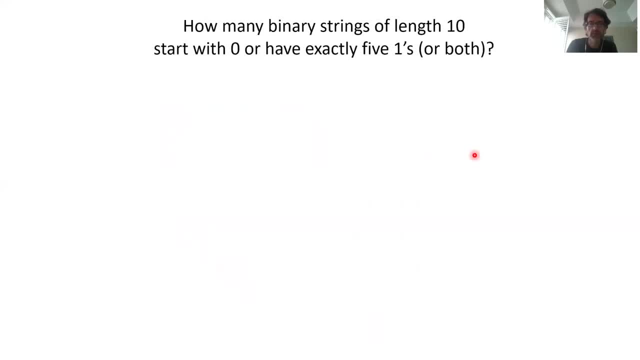 Okay, Some more examples: How many binary strings of length 10 there are that start with a zero or have exactly five ones, or both, Because it's a standard or Okay. So you have two sets: The set of 10-bit strings which start with zero and the sets of 10-bit strings that have exactly five ones. 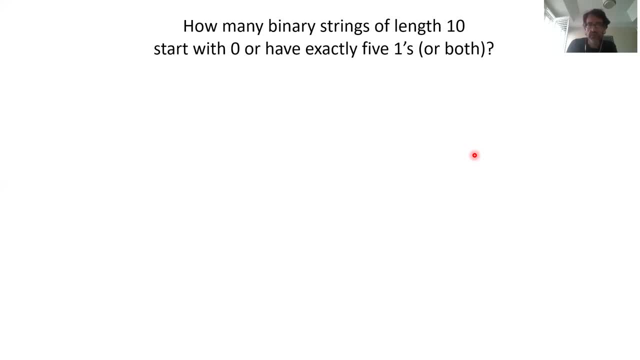 And you note that these two sets intersect. Their intersection is not empty, So you will use this inclusion-extrusion to count the cardinality of the union of these two sets, which is the answer here. Okay, So let's count A1. 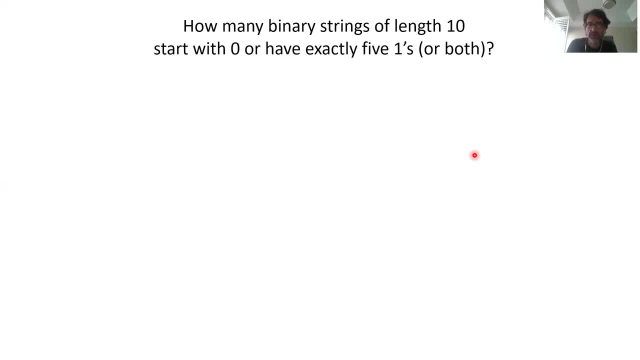 How many strings there are of this type. Well, you fix the zero and you have nine bits that are free, So it's two to the ninth right, Because it's just how many nine-bit strings there are Now. A2.. You have 10-bit string and you choose exactly five ones. 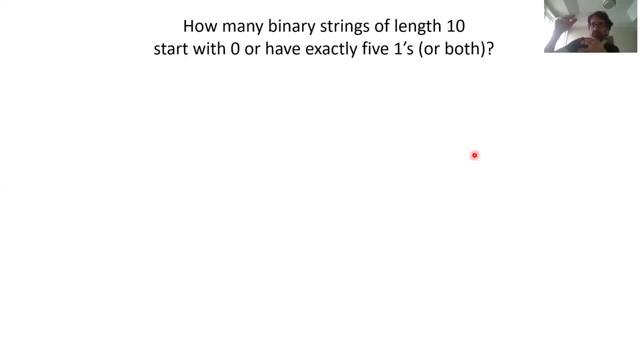 You have to place them somewhere, right. So it's 10 bins with five balls. that are identical. they are ones And the constraint none, No more than one ball in a bin. So you're just choosing five bins out of 10, right? 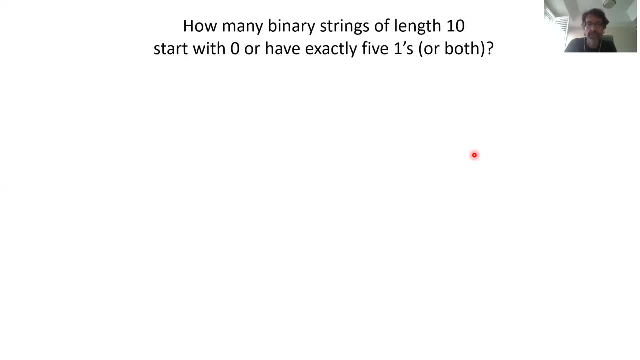 So this is the answer. And now, what about the intersection? Okay, So what is the intersection? The intersection are strings that start with zero and have exactly five ones, both, And that's easier to count than the OR, stuff, right, Because they have to satisfy both constraints. 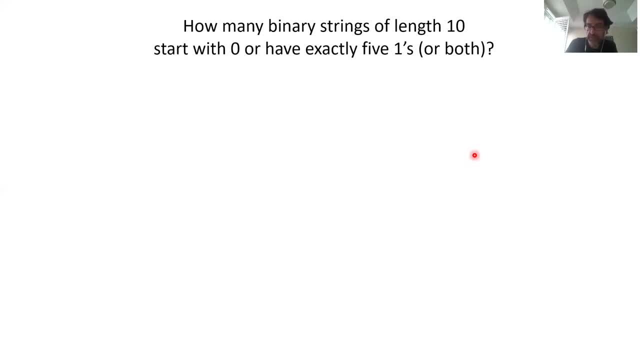 So you fix first. If you first fix the first bit, it has to be a zero by this constraint, And the other constraint tells you that five of the remaining bits have to be ones. Well, there's so many ways to choose five bits out of nine, to place the ones in right. 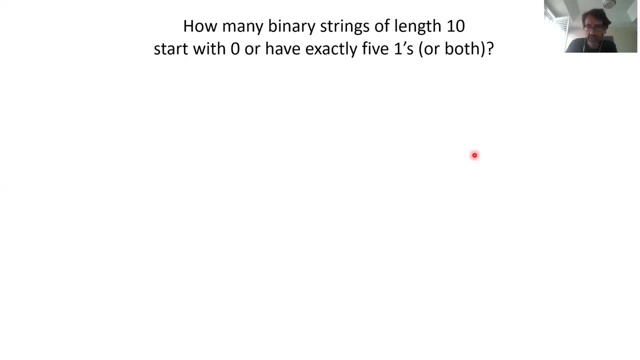 So the general answer is that, Sorry, not again, not the general answer, the final answer using the general formula instantiated here: Okay, How many strings of length six over alphabet ABC have at least five consecutive A's? Okay, The funny constraint. but let's look at that. 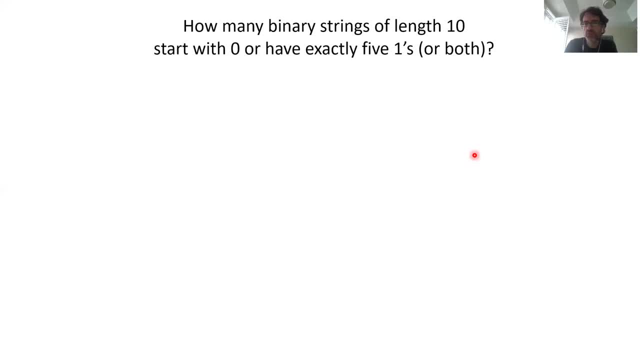 So well, there's- basically there's two sets of these strings. that satisfies this. There are either strings that start with five A's and, because they're of length six, have an unconstrained last character, or strings of this type and they intersect. 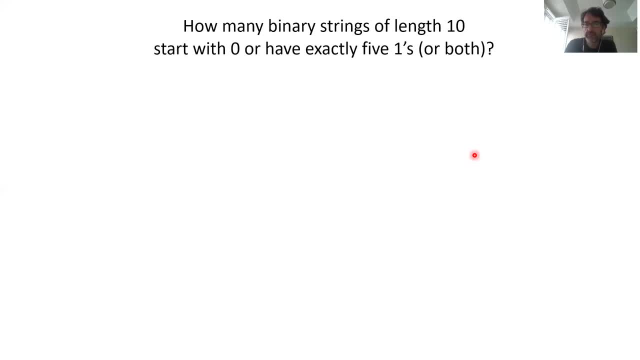 What is the intersection? It's a single string that looks like this: It's both in here and in here. So multiplicity of these individual sets is three, because there's just one character. that is unconstrained right. It can be A, B or C. A, B or C. 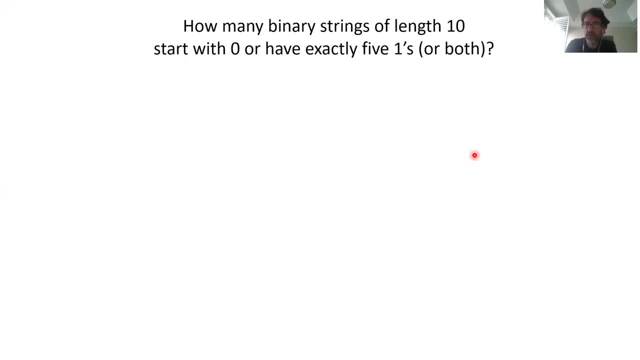 And, of course, this intersection. It's a singleton, It only has this one string in it. So this is the final answer. right, Okay, You can check it by hand. right, Counting these strings. Now, what happens if you have three sets? 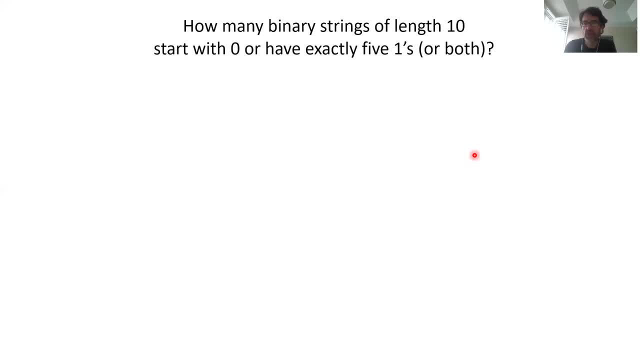 Well, you add them, individual cardinalities, You subtract pairwise cardinalities of pairwise intersection And then you add Cardinality of three-way intersection. Why is that? Okay, Look at these sets. Okay, Cardinality of A is this remainder plus the intersection. 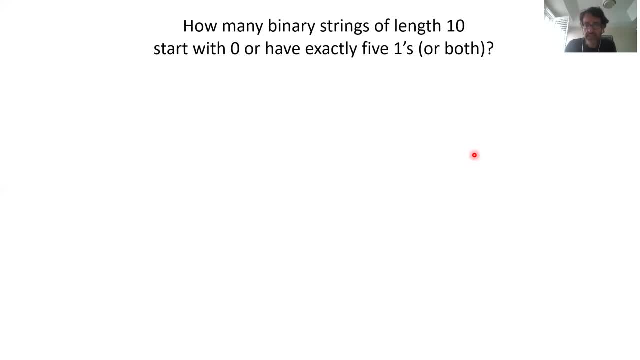 And now intersection with B right, But the intersection itself can be also split. I and X are the pairwise intersection of A and B, But X is the intersection. It's a three-way intersection between A, B and C. So when I count the cardinality I want to count these individual regions independently. 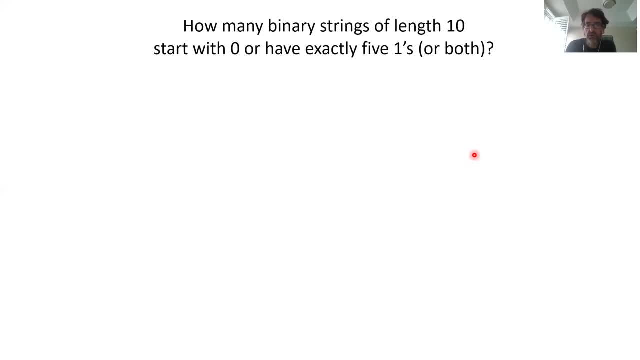 I want to count all the R1,, all the R2,, all the R3, and then all I, all J, all K and all X. But if I count, if I look at the first term by itself, look what happens. 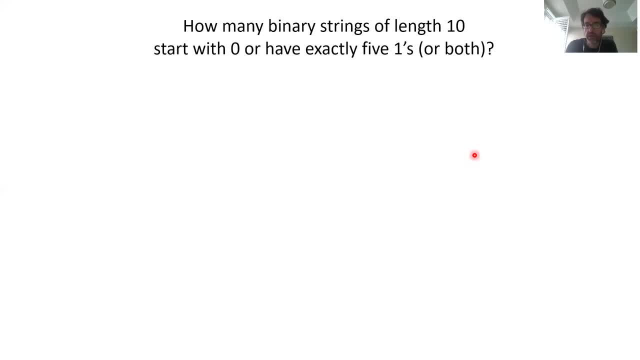 I get R1 once and R2 I get once and R3 I get once. But how many I's did I get? Actually, twice. I got them once as a part of A and once as part of B, And that will be the same with K and with J. 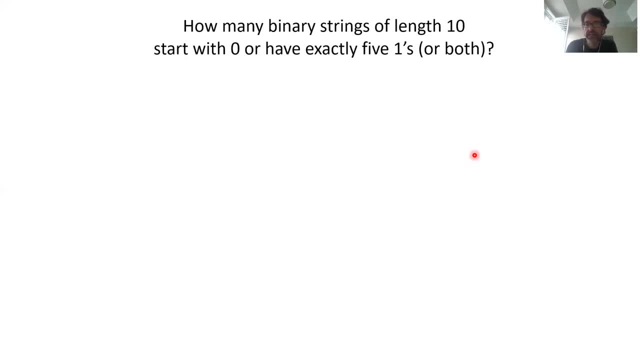 I get all of those guys twice And I get X three times: Once as part of A, once as part of B and once as part of C. Okay, If I correct by kicking out the sizes of these intersections, then what happens? 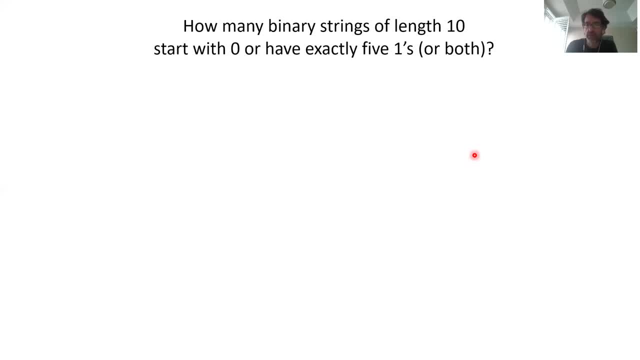 Let's compute the pairwise intersections. Well, these intersections are IX, INX is here and KNX is here and JNX is in the intersection of B and C. So I did count IJ and K once, but again I counted X three times. 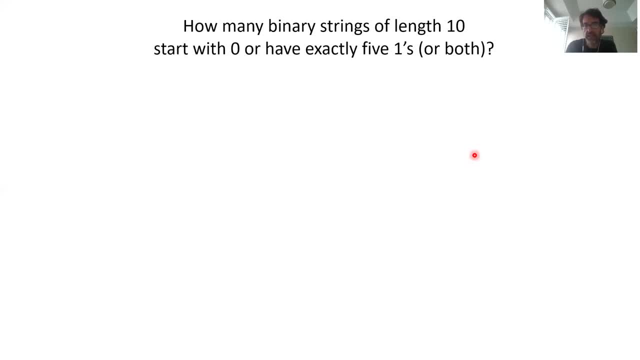 So if I just take this thing, which is this one- pairwise intersections, cardinality of pairwise intersections- I would correct this part. so instead of 2, i plus j plus k, I will have 1,, because I would subtract this part, but I would kill off x. There will be no x, That's why I have to. 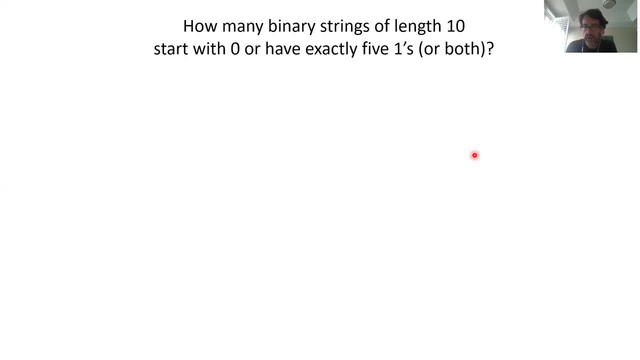 add this back. And now, when I take s1 minus the pairwise intersection, plus the three-way intersections, I get the correct thing. Okay, And if there is more sets, then the signs will just alternate, And if there is four sets, then I will subtract. now I will. 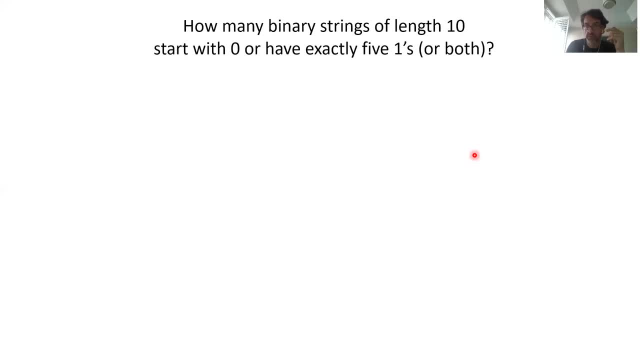 have here all the three-way intersections, which there will be four possible ones for four sets. Pairwise intersections for four sets will be 4,, 2, 2.. And finally, I will subtract the pairwise, Pairwise, the all four-way intersections, And if there is five more, I just have more. 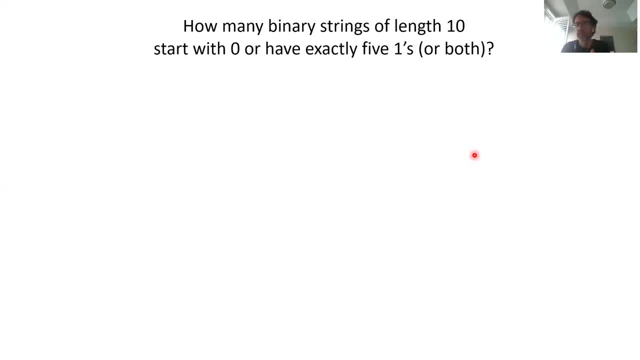 of these, I add, I subtract, I add, I subtract the next k-wise intersections And then k plus 1-way intersections. I take with an opposite sign. Okay, Let's see some examples. So say you have a drug test on a population of thousand. 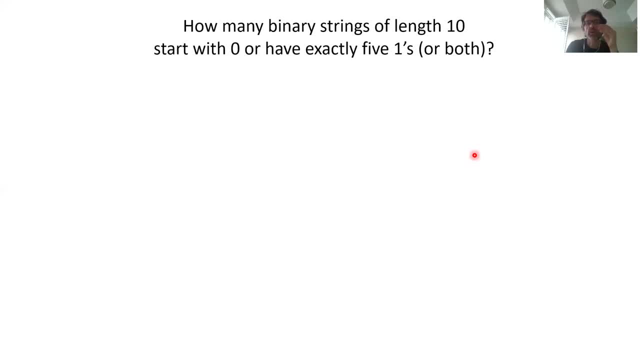 people And there's three symptoms: A, B, C, three different things. you test, Okay, Three symptoms, you observe And you told that cardinality of first symptom is 122.. Second 88,, third 112.. But the pairwise cardinalities are also given And the three-way cross-section is: 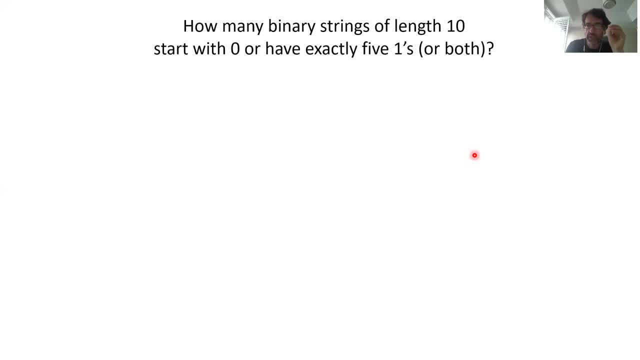 also given, And the three-way cross-section is also given. So you can use any of these formulas, but what now? Okay? So the second point, of course, is that you already know which symptoms occur, That there was so many people were in the intersection of: has a symptom. A- has a symptom. 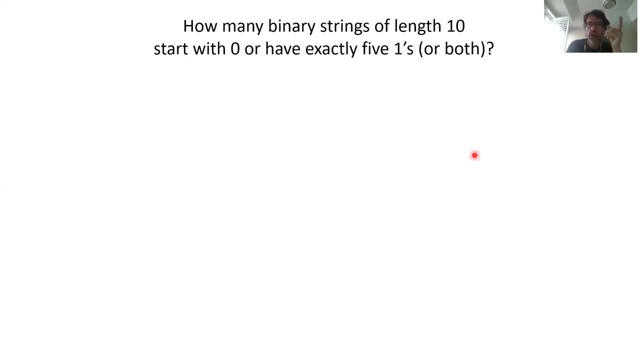 B and has a symptom C sets. So how many people are there in total who got any symptom Right? It's the cardinality of the union of A, B, C And we can count it because cardinality of the union is the cardinality of individual sets minus cardinality of pairwise intersections. 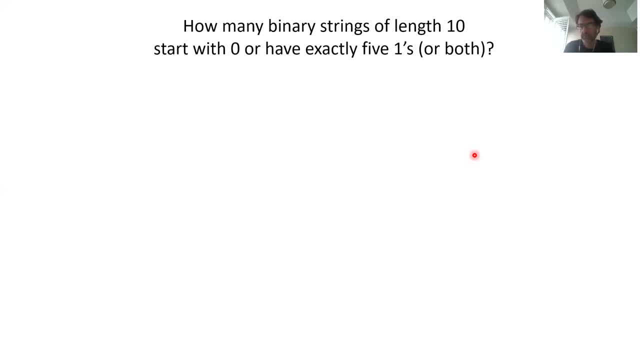 intersections plus carnality of three-way intersection. so, given all these numbers, we can exactly compute this right. it's as if, uh, we were told here what is the total a, total b, total c, and we're also told what's the total k plus x, total i plus x, total k x plus j, and as we're, 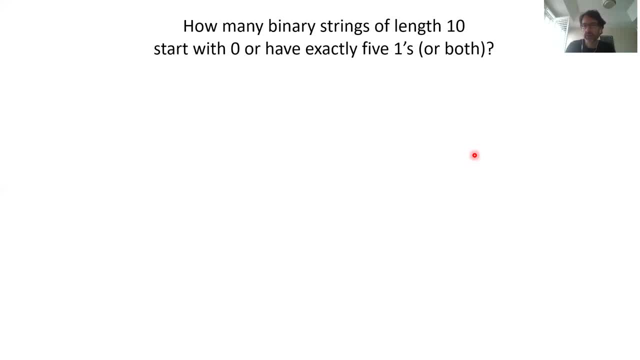 told what's x. well, that fixes all of these variables, so therefore, we can compute it right using this formula. we have enough data here, okay, uh, so here is a more- i mean okay- an example that relates to some other counting problems that we have done, so let's look at it. 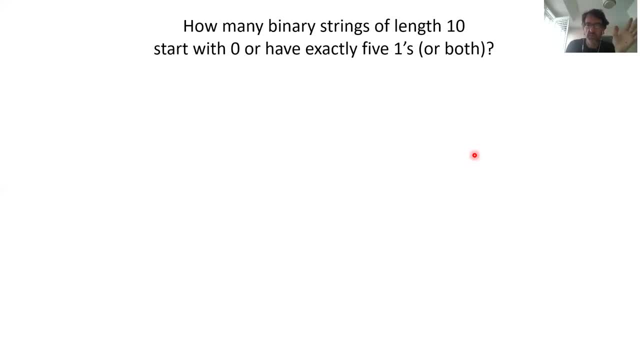 because, even if we don't have exactly this problem, but it's still about counting um people like people like line lined up. so let's say you have seven people: mother, father, three sons, two daughters. how many lineups of this family are there where mother is next to at least one of her three sons? 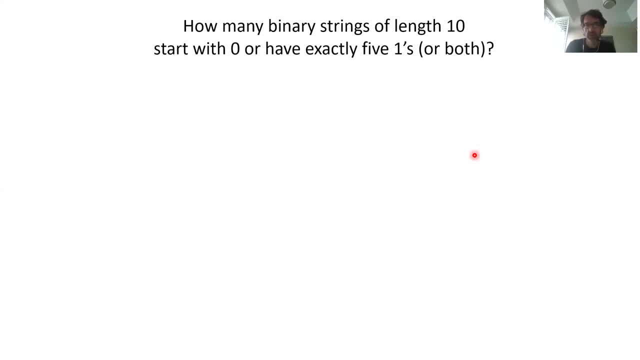 okay, so let's have these three sets to be said, ai is a lineup where mother is next to son i. these sets could intersect because you could be next to son one and next to son three. uh, so these are the pairwise intersections and, uh, well, i can still write this expression right, the intersection of three sets, but this: 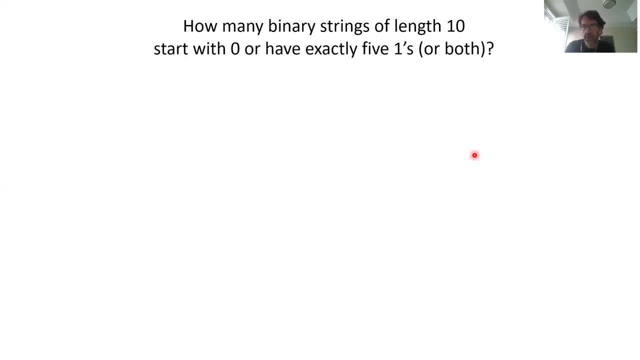 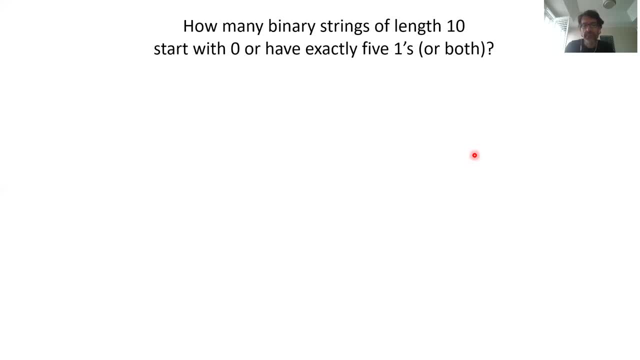 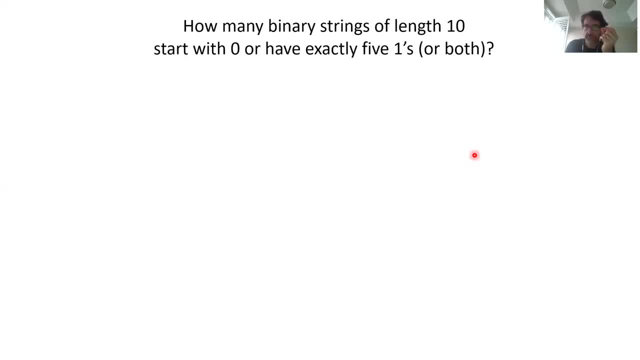 they line up right. so it's son, followed by mother. that's why i'm taking two of these permutations over six elements. now, what about? mother is next to both sons. well, here are the possible solutions. let's treat son i, mother, son j as a unit, and let's treat s j, m s i as a unit. either case is. 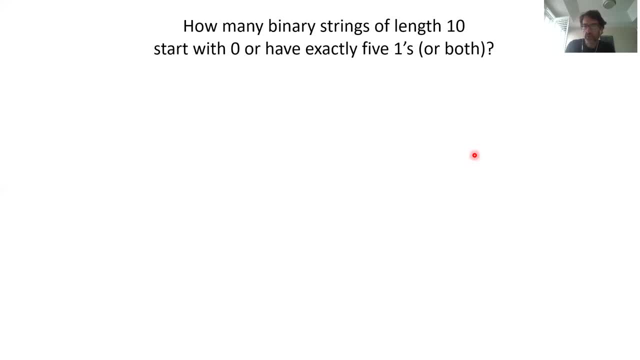 a problem. or now you have this extra unit where three of the seven people became one unit, right? so how many units? there are five, right, it's the four remaining people and this conjoined, monstrous entity of a son, mother and another son. you always walking, you know. conjoined, right? so it's five factorial and there's two of them because 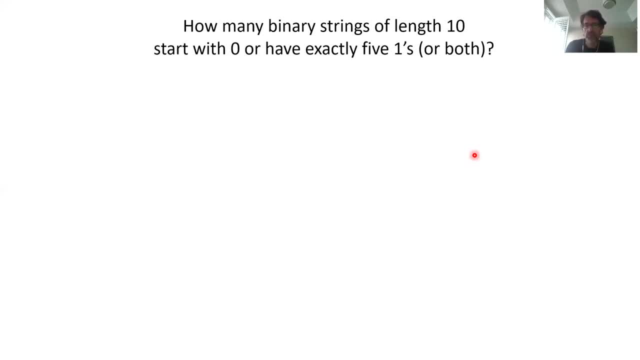 one using this unit and one using that here, right, and the three-way intersection, as we said, is empty. uh, so this is your final answer, right? it's three of these, so it's two six factorial. two twice six factorial times three. it's three of these, so three times two, two times five factorial. 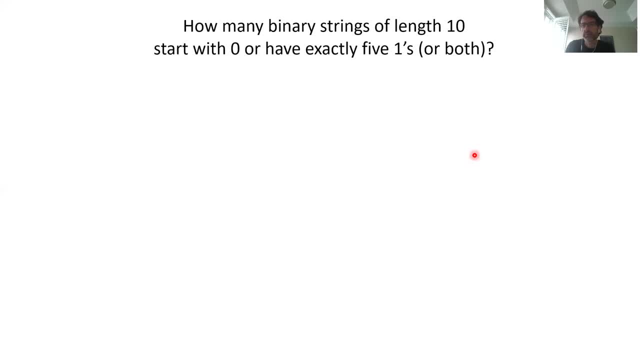 so it's three of these. so it's two, six factorial two twice six factorial times three. uh, so it's three of these. so it's two, six factorial two times three, and uh, well, it simplifies through to that, if you want. okay, uh well, here is another, uh, more general, even more general example. so 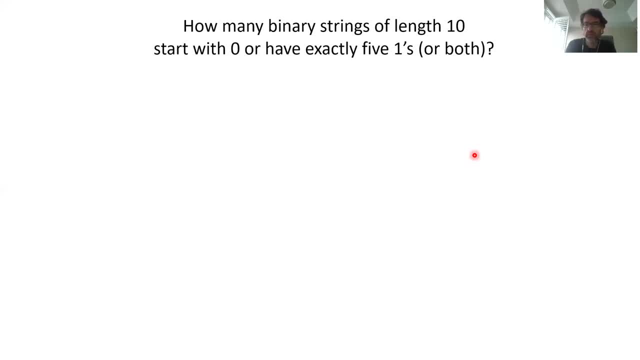 have, uh, at least four consecutive a's. oh, okay, sorry, sorry, no, this is not so hard, but okay. so there are three. these are the three sets, um, um, um, you can. these are the pairwise intersections and there is a three-way intersection, and the ways to count it right is there's six square of these and six square of these and six square of. 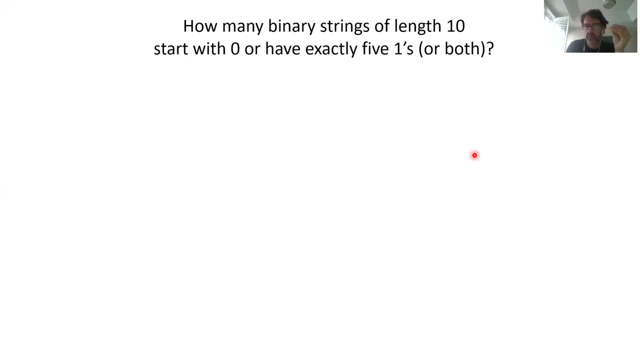 these, because it's an alphabet of six and there is two positions, so each of them is six square and there is three of them. so, boom, you have that these are six of both of of this, six of these and one of these. right, look, they're asymmetrical because if i intersect this set with this set, 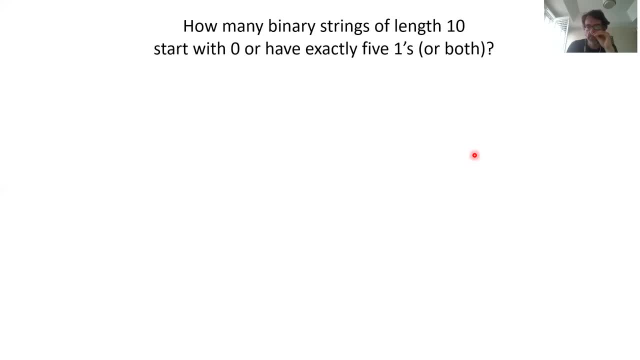 i get only one string always, and there is something in the three-way intersection. right, it's that string again. so you have to kind of be clear about this. it's hard to do this all in the head. you have to write out these things, count them by the book. 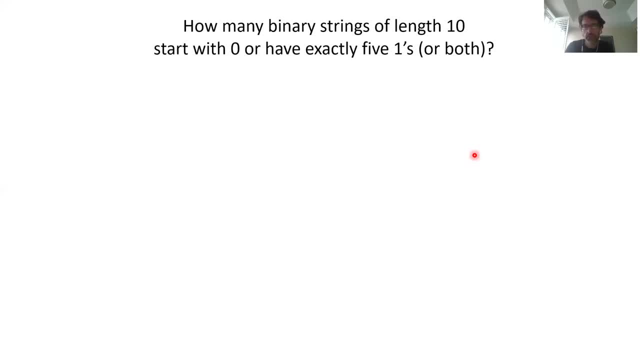 um, otherwise you're likely to make a mistake. um, here is a very sweet application to prime, to counting primes in a way. so remember primality choice like. well, we could choose a problem by like okay, let's eliminate all, let's okay. or test primality, how about you eliminate all? 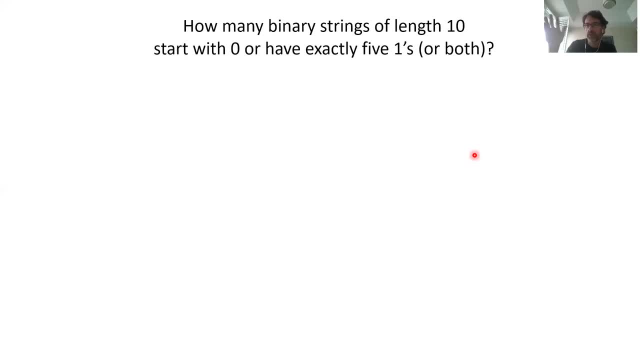 you, you, to eliminate all by three, by the next prime, and so to write how many elements in a range you eliminated, how many are left, and these will be primes, right. so let's do it in a limited way. let's just eliminate just multiples of two, three and seven and let's count how many in this. 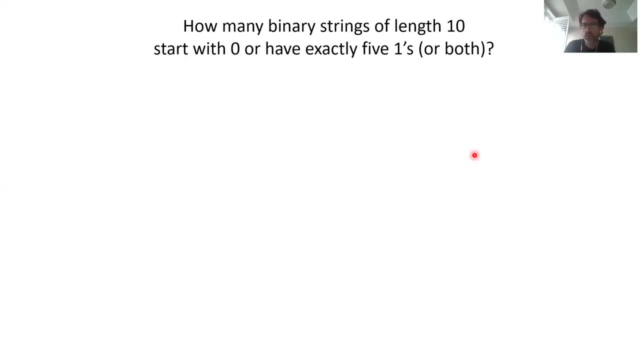 arbitrage range are already kicked out by what i've done. what, um, what is now? but like this: right, these are not all the primes here, right, right, because i should also kick out multiple pieces, five of 11, 13, yeah, yeah, yes, because all of those multiplicities will be here. 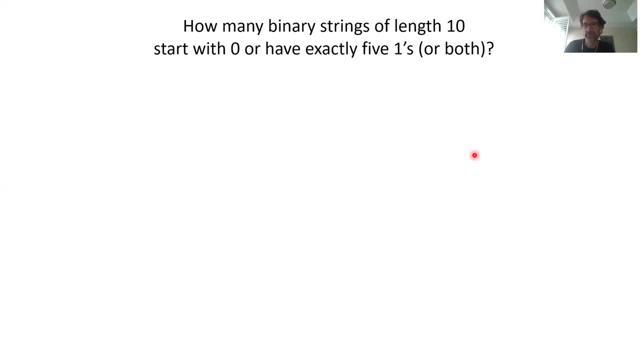 uh, well, okay, some will be, will be now. um, yeah, but fives, i should definitely kick off, right, um, so okay, uh, let's, let's, let's look um. so A1 is 3.5, let's add 3.5. Arkansas옵 is 3.5. 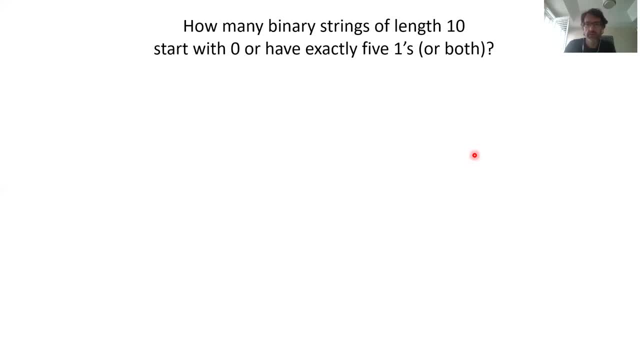 let's add 3.5, right, grandpa? some aumento. let me, at 16, at a 1, give back 2.0 and 2.0. this should have been up by 75.2.. set of elements that are zero modulo two and a two is all those that are zero modulo three. 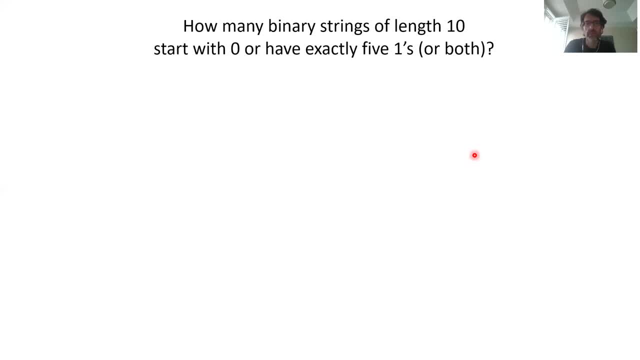 and these are zero modulo seven. uh, the intersection. there are zero modulo both two and three. there are zero mod six, the residue. well though, okay, i mean, how can a number be both divided by two and by three? this number must be divisible by six. how can a number be divisible by two and by 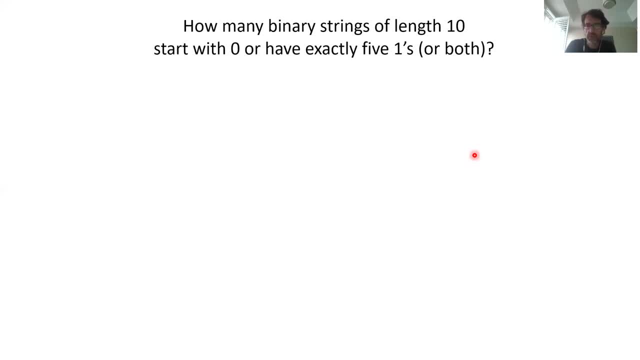 seven. it must be divisible by 14, so it's zero mod 14, and both by three and seven. well, it's zero mod 21. um, and the intersection is just zero mod 42, right, because it has to be divisible by two, three and seven. if i multiply them is six times seven is 42. 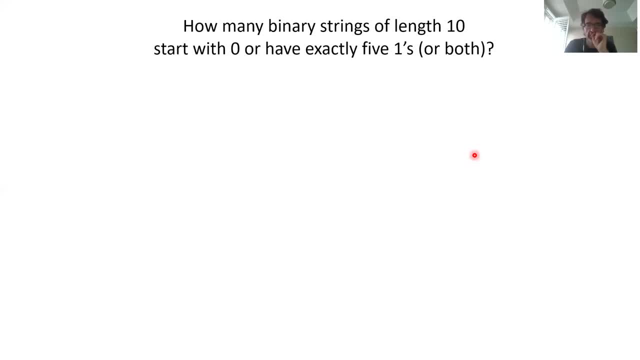 you. so, um the those which are by, one of them is those which are in the union of a182a3. and how they count the size of this union: inclusion, exclusion principal. i add the cardinalist of individual sets, i subtract the current of pairwise intersections and I add the commonality of three-way intersections. 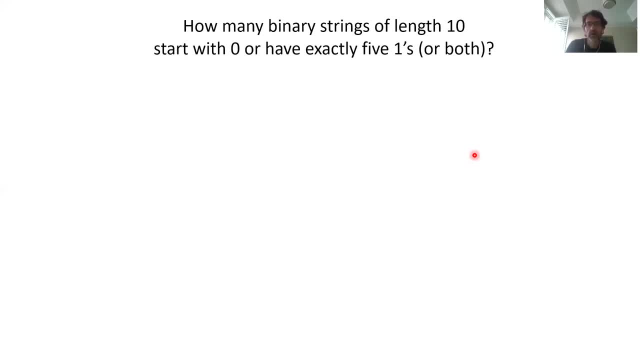 So the number of elements in here at the number of those which are 0 mod 2, so it's every other, so it's 42 divided by 2.. Those which are 0 mod 3 is every third, so it will be this many. Those which are 0 mod 7, this many, and so forth, right, 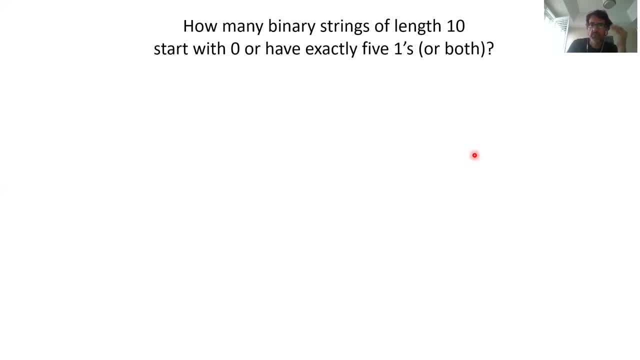 Because this is like- if this is how I define the problem, it's just, it's clearly like the ones who are 0 are every sixth or every fourteenth, and I chose these numbers so that 42 has a round multiplicity of either of these. 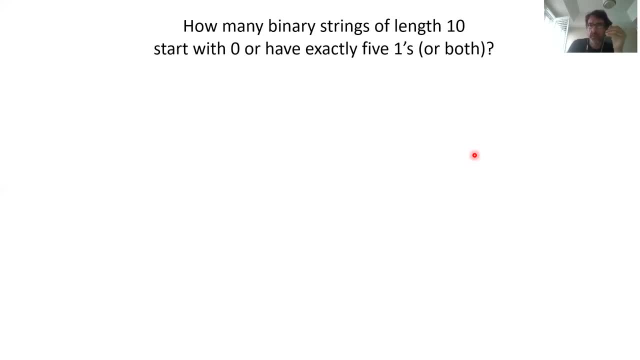 factors and therefore also their products, So that you don't have to do ceilings here at any place. right, Exactly All of these are integers And triple intersection. in this range, the only guy who's 0, mod 42 is 42.. 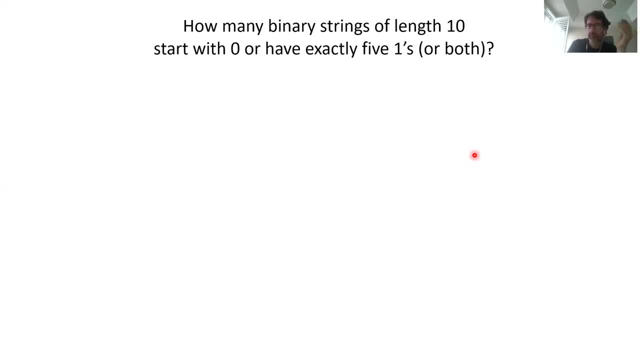 So I only add 1.. Right, so I add these subtracts, these pairwise, add the triple and I get 30. So majority of Flash, this interval, right? Well, half the interval is divided by two, right? But here you know. 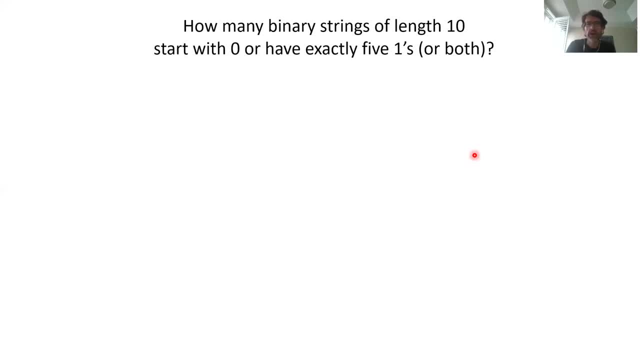 this fraction exactly, And if you have a four-way intersection, right? so if you were counting cardinality of a four union of four sets, you add the individual cardinalities, you subtract pairwise cardinalities, you add three-way and you subtract four-way, and that's how it would go. 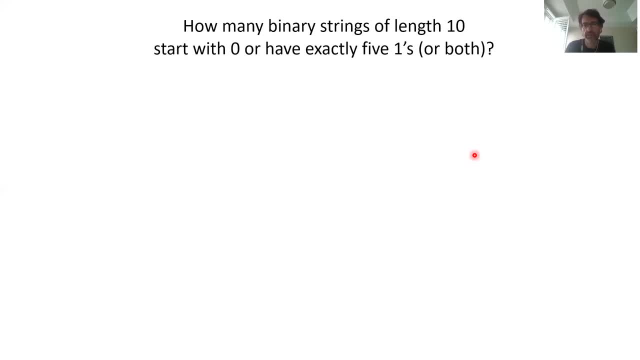 for larger, You can see how it generalizes. So let's take elements. the sets have 15 elements, but you are told what are the pairwise intersections and you are told what are the three-way intersections- cardinalities, and then also you told the four-way intersection. 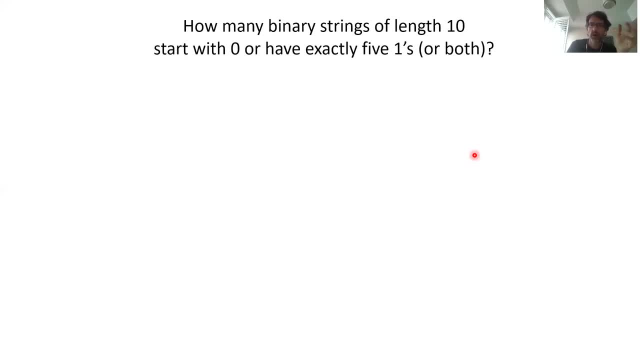 And now you ask: well, how many of these elements are there? So if these intersections were all empty, then you would note that the set of elements has 15 elements. the total number is 60, 15 of all the sets, but they're not empty. okay, so what's the size of the?